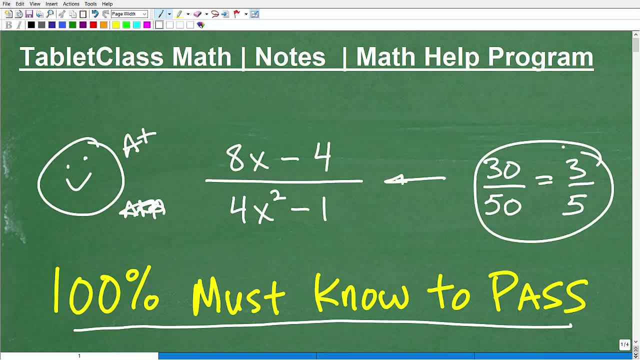 great skills in this particular area, And what I've found is that a lot of students struggle with this And if they correct, if they get really good at this category, this kind of subset of algebra, everything will go much, much better for them. So I'm going to get into what this is And I'm going to give you some specific advice on how to improve in this really extremely important, vital algebra skills. We're going to get to this in just one second, But first let me quickly introduce myself. 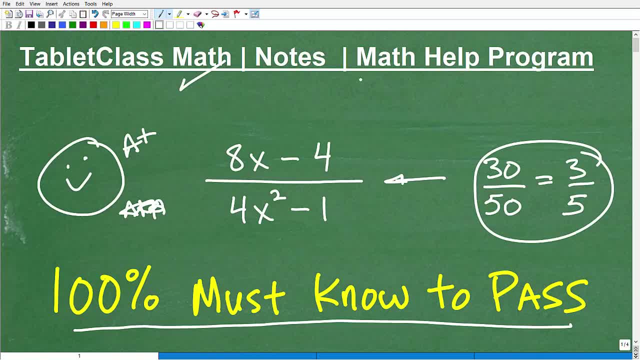 My name is John. I'm the founder of tablet class math. I'm also a middle and high school math teacher And over several years I've constructed what I like to believe is one of the best online math help programs there is. Now, of course, I'll let you be the judge of that. If you're interested, you can check out my math help program by following the link in the description of this video. But basically I have 100 plus different math courses, ranging from pre algebra, algebra one, geometry, algebra two. I'm going to be launching pre calculus here literally in about a week, So if you're into advanced math, you might want to check that out. 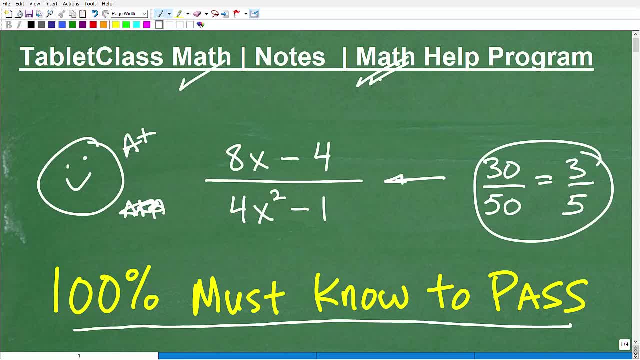 Check out that course, But I also do many, many or have many, many courses in the area of test preparation. So if you're studying for, like the GED, HiSET, TASC, SAT, ACT, GRE, GMAT, ASVAB, ACCUPLACER, CLEP exam, ALEKS exam, maybe a teacher certification exam like the CBEST or Praxis, There's a ton of exams that people have to take for all kinds of reasons. Okay, it's not just school. maybe you're getting into a program, maybe you're trying to get a certification. 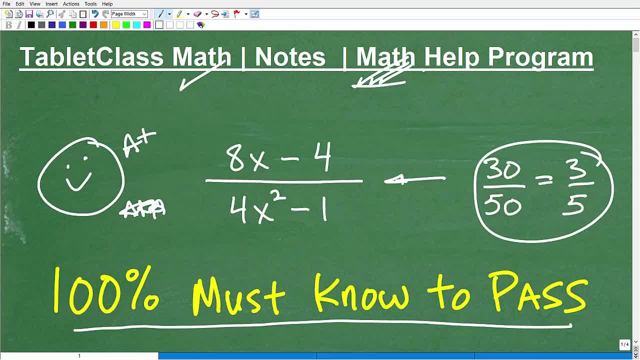 For whatever the case might be. but all these exams have one thing in common. That is math, And if you don't do well in the math section, you do not do well on the exam. So I can help you out to prepare to be successful in these exams. Just go to my website and check out my full course catalog. If I don't have your exam, okay, drop me a line and I'll help you out the best I can. I also do a lot with homeschooling, So if you homeschool, I have a great homeschool learning system And then, obviously, help those of you who are having a tough time in your current math course. 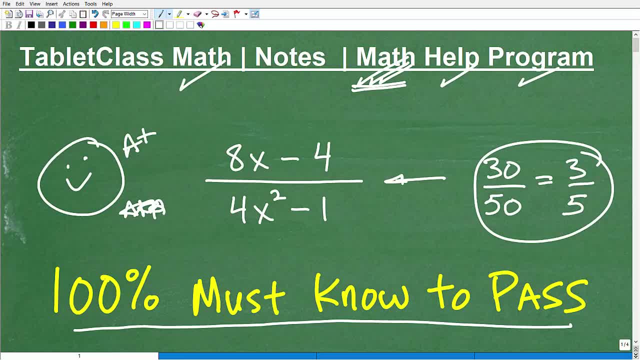 Now, if you truly are serious about wanting to improve in math- and if you're not serious, then just disregard this. But if you are serious and you're watching this video, you know you're probably interested in getting better at math or learning math. But if you are a student, you got to be serious about taking notes. Now, I've been teaching math for decades And there's one thing I can always point to with consistency, And that is those students who take great math notes almost always end up looking like this at the end of the school year, And the reverse. 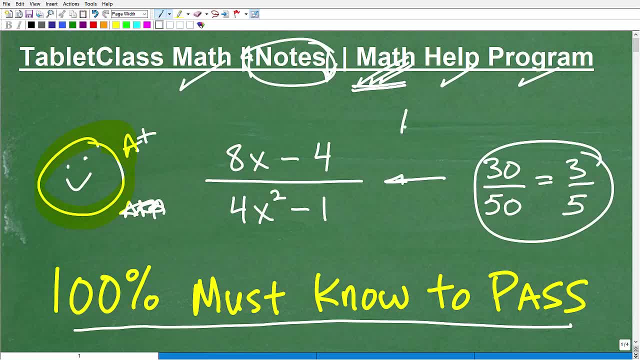 is true, Those students who kind of blow things off, kind of like how I did back in the good old 1980s. I wasn't a great student, I definitely wasn't focused And I was trying to cut corners every which way I was taking notes, but they had nothing to do with math, They were like back and forth: Hey, what are we doing this weekend? And we're doing this because we didn't have any cell phones. If I had a cell phone back in those days, I don't even think I would have graduated. So you got to really focus on being focused. That requires work and discipline, But if you can remain focused, 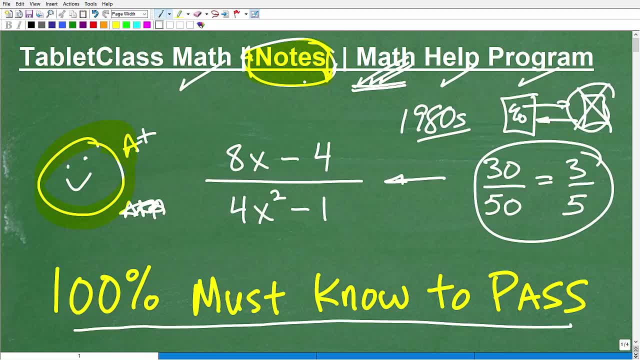 and engaged and write that information down, don't. I'm telling you right now. so many out there think that you could just look at the teacher teaching without writing things down. That's not going to be good enough. You have to physically write things down on your paper: neat, organized, detailed. that's going to pay off big time. Okay Now, as you're improving in your notes, you can use my notes to study from. So those will include pre algebra, algebra one, geometry, algebra two and trigonometry. You can find the links to those notes in the description of this video. 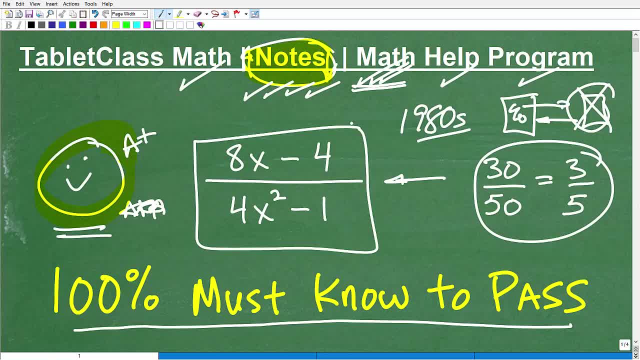 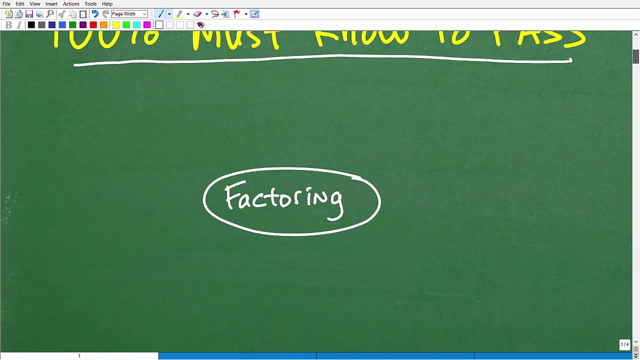 All right, now let's get to this problem. If you think you can do this problem and simplify it, go ahead and do so. I mean, this is not, let's just say, there's many, many other type of more challenging problems. This is actually pretty easy to do. But if you can do this, you want to just challenge yourself real quick. Go ahead and, you know, pause the video and do the problem, because I'm going to do this here in just one second. But let's get to what I'm talking about. And there it is. I'm talking about factoring. Okay, So many students. 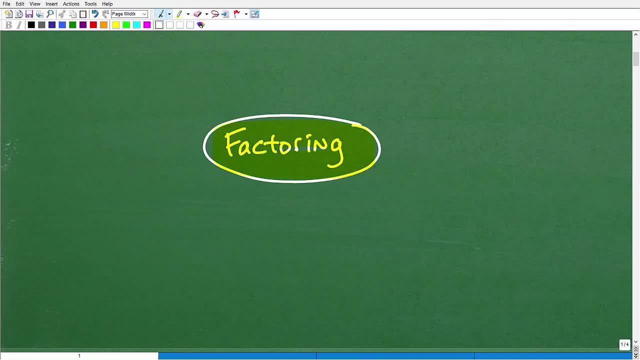 are not as strong in factoring as they really can be or need to be. Okay, If there is one skill, that in algebra that I would say- and there's so many different skills are important, but I would have to rank this up here, Maybe like the number one top skill for you to go and invest in that will make your life easier. Now, what are we talking about? Well, we're talking about factoring with the greatest common factor. Okay, so things like this, Can you? 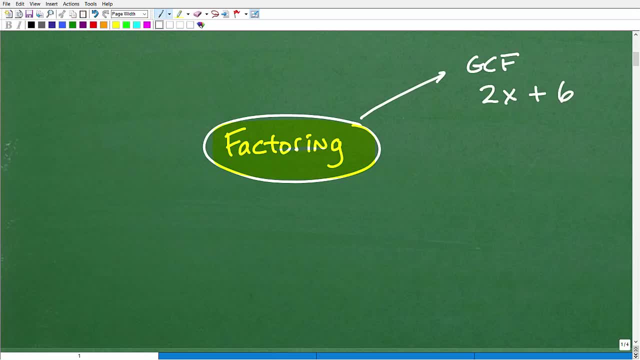 factor, something like that. Now, what does that mean? Well, it means to take out the greatest common factor, right? This is an illustration of factoring. Okay. so you always start off with learning how to factor with the greatest common factor, And then you get into working with trinomials and stuff like this: x squared minus one, x plus two. this, right here, I don't even think is a factible is a factible here. Let's just do this real quick: Two factors of two that add up to 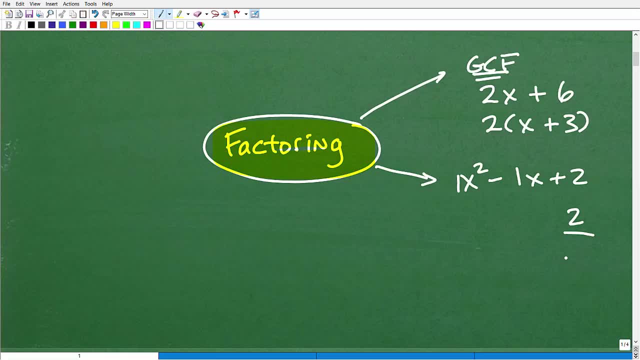 negative one. Nope, it's not factible. Okay, So, anyways, you start off learning about trinomials And then you get into this is the basic trinomial. then you get into things like this: All right, So you're. what we're trying to do is to determine whether these things are factible. So let's take an example of a number. is this number 10.. Can you factor this number 10?? Well, yes, it's two times five. it's not a prime number. 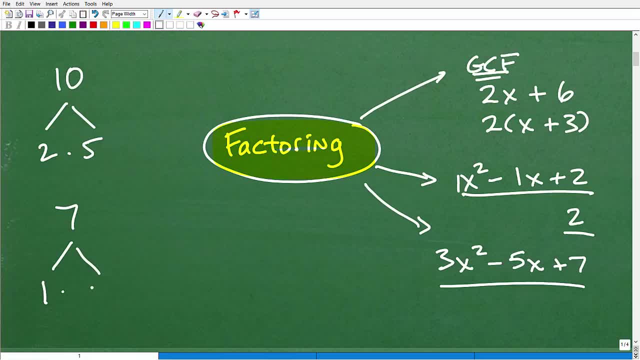 Can I factor seven? No well, I can only factor with one. So this is the definition of prime. So not everything's factible. So we have all types of things in algebra that we can't factor, but we don't know that until we really try to factor what we're dealing with. So dealing with trinomials is huge, Okay, but you have to first start off by mastering the greatest common factor And then, after you've done all this, then you get into special factoring rules, special 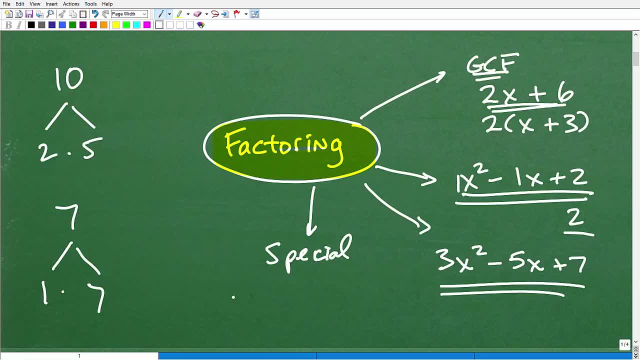 special. Let me see here, make sure I can spell that right. So this would be like x squared minus four And that's equal to what x plus two times x minus two, difference of two squares. There's all types of other- well, not all types- And there's group factoring. So factoring is a huge, huge skill. You need factoring to do a wide variety of problems in algebra and to learn a wide variety of topics. If you cannot factor, you're literally. 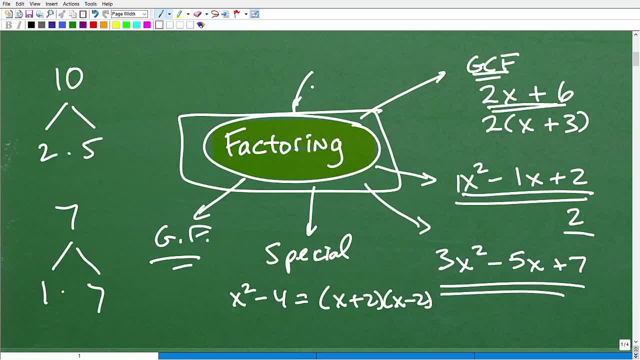 not going to do it, going to be able to do a ton of the chapters in algebra and that's probably going to result in you not passing. so I'm not really exaggerating when I'm talking about this and what I've seen over the years is students kind of know a little bit of factoring but they struggle, they never. 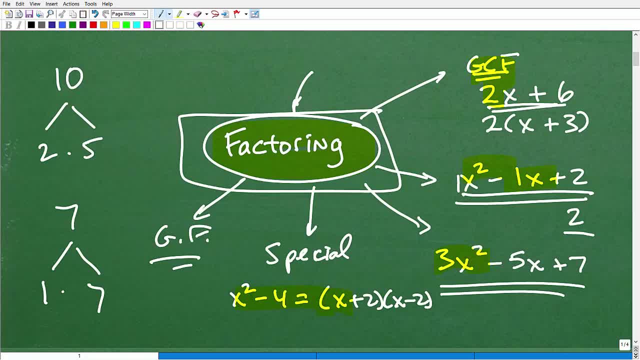 really picked it up. so let me give you some quick suggestions on how you can improve in factoring. first, okay, I have tons of videos on factoring in my youtube channel in my algebra pre-algebra playlist. okay, so that's the first thing. on various different factoring topics also, you 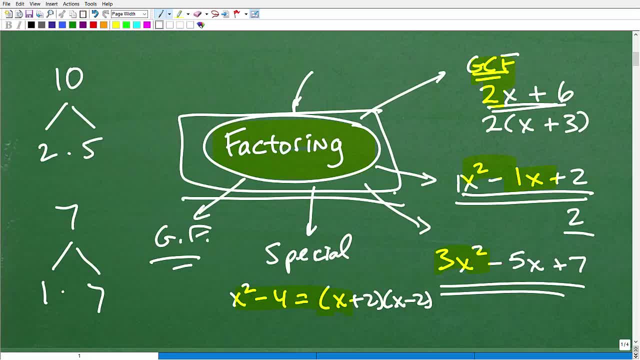 might want to consider checking out my algebra, one course where I teach this extensively, but I would always start here with the greatest common factor. make sure you understand how to do the greatest factor out, the greatest common factor. so this is the reverse of doing the distributive. 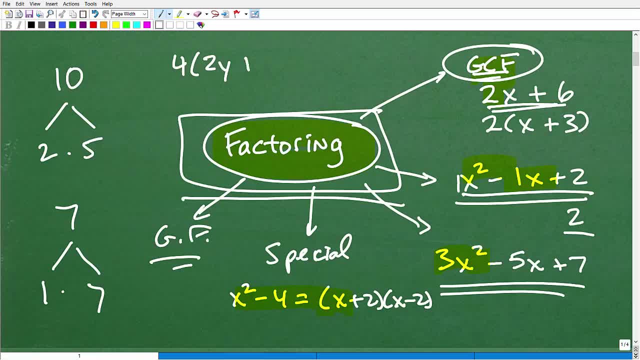 property. so if I have like four times two y plus one, make sure you can multiply. probably here a lot of students mess up the distributive property. this is a y plus four. okay, now what I've seen over the years: a lot of students, when they don't understand this enough, they'll go: oh this. 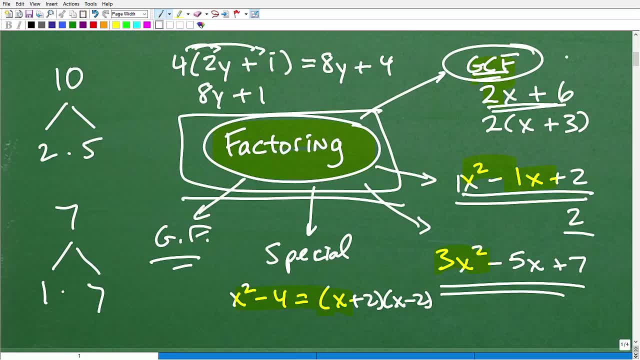 is a y plus one. they forget to multiply over here. so when you're looking to improve with the greatest common factor, make sure you understand the distributive property really well, because factoring is the reverse of doing multiplication. so start here, okay, make sure you're really really. 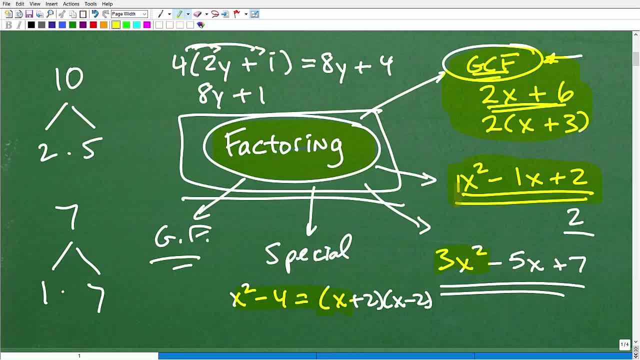 good with this, and then start with the distributive property, and then start with the distributive property, and then start with the easy trinomials where the coefficient of the x squared or a squared, or whatever it might be, is one. master these and then move on to these and then finally go to into special factoring rules. 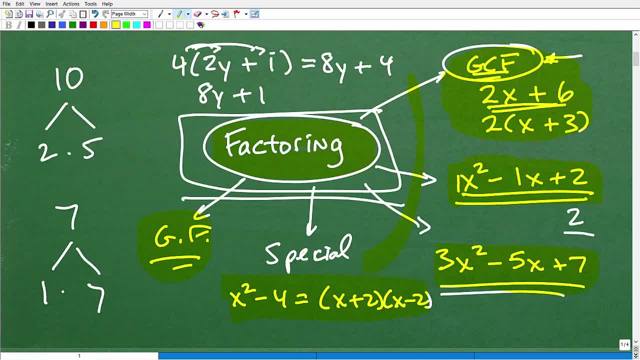 and then learn more about group factoring. but you got to know all of this stuff and, again, this is absolutely one of these things that if you don't know it, you literally cannot do the problems okay, and there's a ton of problems in the algebra that require factored skills. so, anyways, hopefully this is kind of set up some sort of game plan for. 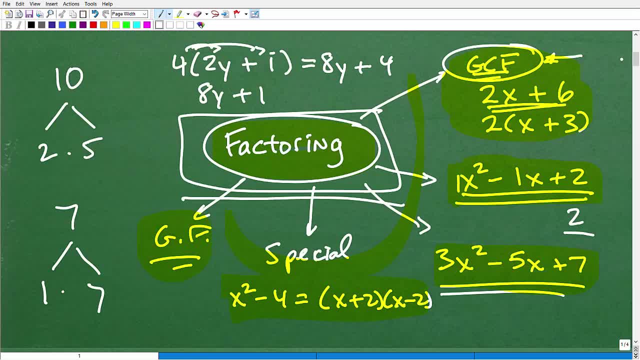 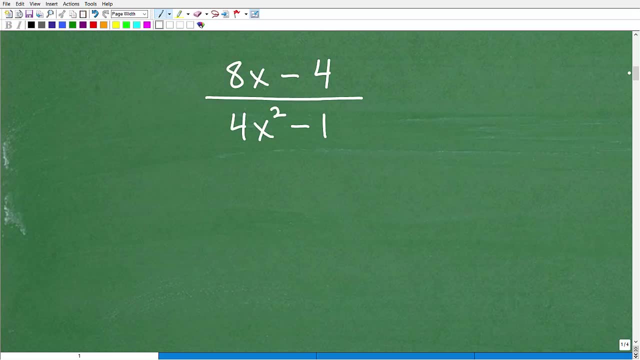 wherever you might be, but this is definitely worth your review. okay, just validate that you're super strong in factoring. if you are, things are going to go pretty smooth. but now let's get into this problem right here. so let's simplify this now. I could have done a lot of. there's a ton of different. 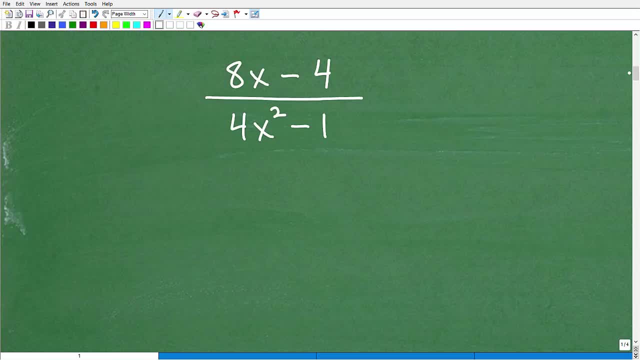 factoring problems, I could do, but I'm only going to do this particular one. so let's go ahead and do it now again, if you don't want to see the solution, okay, quite yet. you want to try it on your own, then pause the video and do so. but let me go ahead and do this now. so to factor, well, let's. 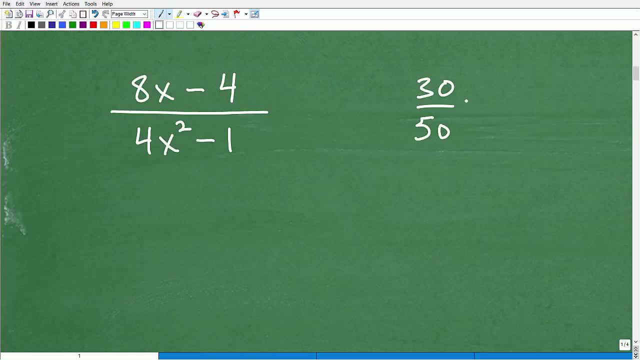 just do this real quick. remember when we had 30 over 50? so I said: oh yeah, this is three-fifths. but really, what you're technically doing there is you're, you're, you're factoring, you're going: oh, that's not three times 10 and this is five times 10. now a lot of you are like: I can cross cancel. 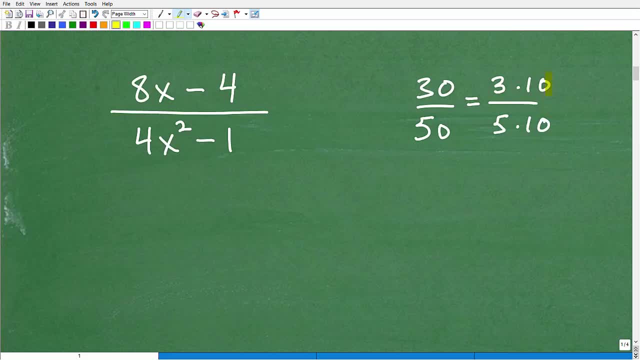 the zeros. but really, what you're doing is you're going to do this and you're going to do this, and you're doing is you're factoring and then you're getting these common factors. okay, this is a factor and this is a factor and we have this fraction, so I could cross, cancel common factors and this. 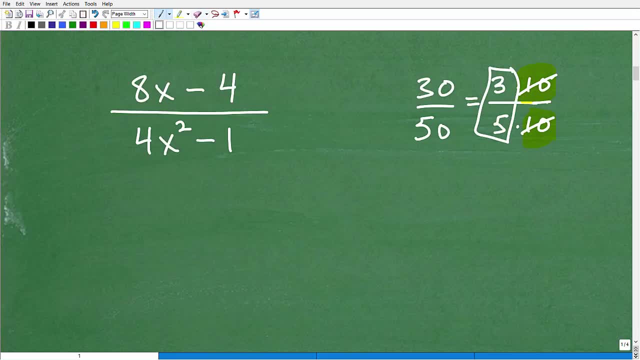 is what remains. so tech, that's the technical mechanics of what's going on when you're simplifying. but we need to understand that because this is what we need to do here. so if I can factor and then go look for common factors, I can cross, cancel them all right. so let's take this guy right. 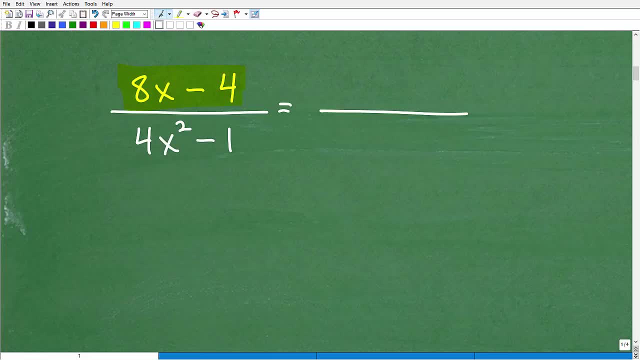 here. this is an example of factoring with the greatest common factor. I can factor out a. what I could factor out a four. nice, so this would be four times two x minus one. now just to double check myself: the four is the greatest common factor. if I multiply back in four times two x, I get my eight x back, and then four times this one. 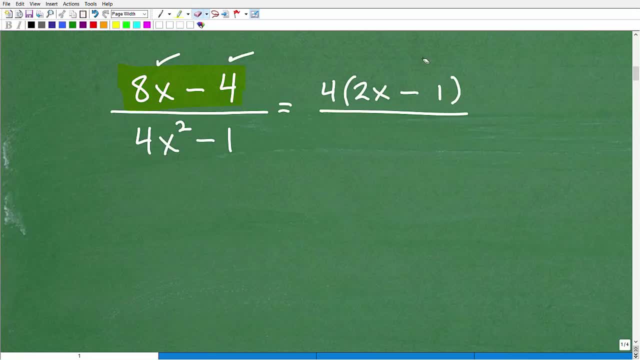 I get my four back. so if you're ever in doubt in terms of whether you factored something correctly, all you have to do is just look at your factors and then just do a quick multiplication and again and make sure you can get back to what you started off with, right. okay, now how about this guy? 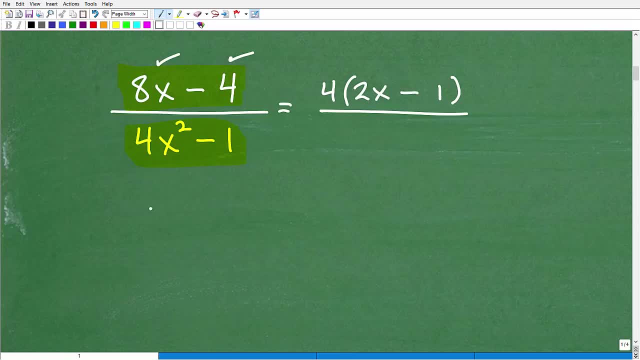 well, some of you are like: well, there's no greatest common factor. I can't do anything like that wrong. this is a difference of two squares, a squared minus b squared. this is a special factoring rule and I don't want to turn this into a whole lesson on factoring, because 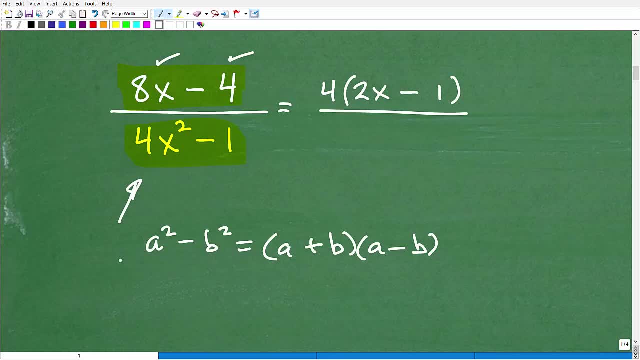 it's a huge topic, okay, but this is basically the rule that you need to know. so this four x squared, I can think of that as two x squared, and then I can think of that as two x squared, and then I can think of that as two x squared, because two x times two x is indeed four x squared, and then one. 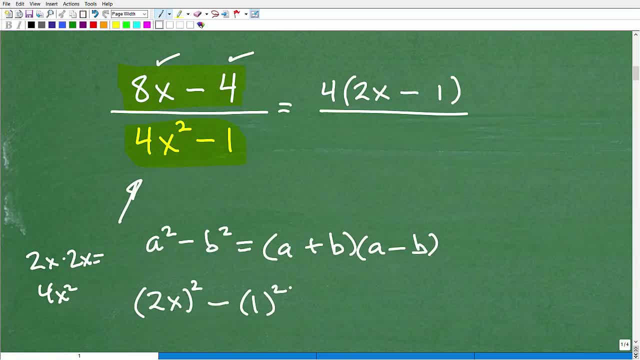 okay is what? well, that's just one squared, okay, so I can think of this one as one squared. now I could just follow the pattern. so this thing is going to be equal to two x plus one times two x minus one, and if you weren't sure about that, you can use the foil method to go ahead and 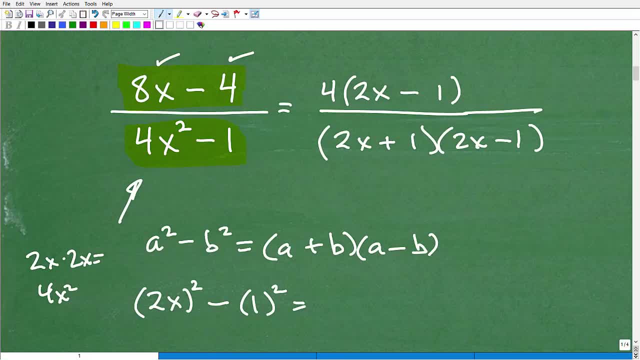 multiply. okay, I'm not going to do it here, but I can multiply all this together and I would get back to four x squared minus one. okay, so now that I was able to factor out both the numerator and denominator completely, now I'm going to go look to see. hey, do I have any common factors? I'm like 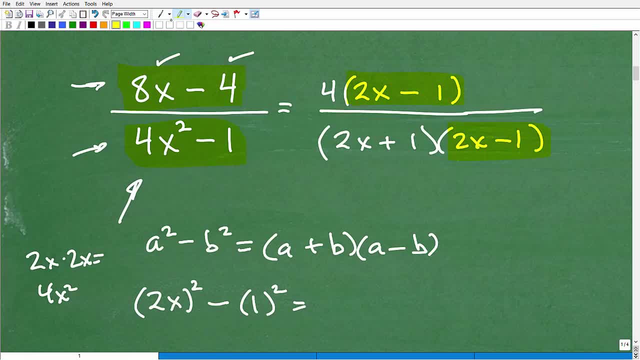 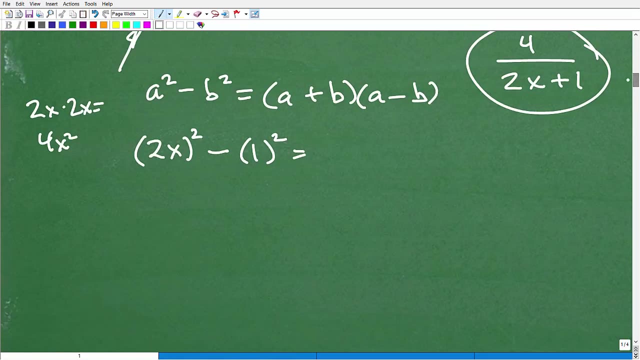 I got a two x minus one. oh look, I got another two x minus one down here. these are factors, so I can go ahead and do this, and so I'm left with. this is my final answer: four over two x plus one. okay, now, if you got this answer correct, then I must give you an awesome happy. 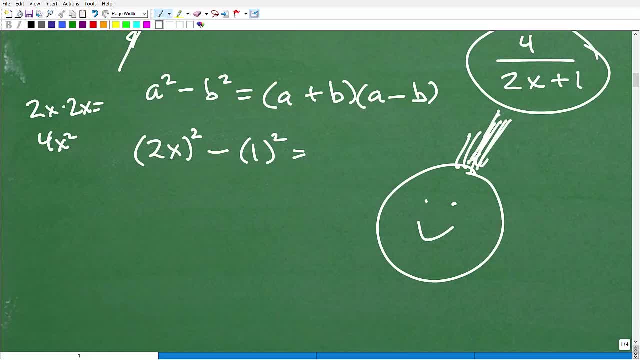 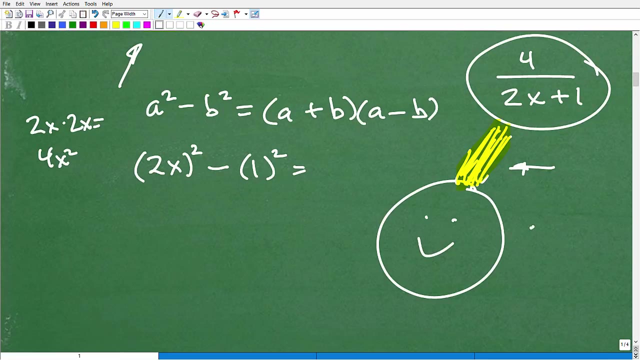 face with a 1986 special mohawk with extra hairspray. I don't know what it was about the 1980s, but we were crazy with the hairspray and, yeah, I'm glad that it's not around because it was probably not the safest hairstyles to have. but anyways, you definitely earned yourself an a plus. 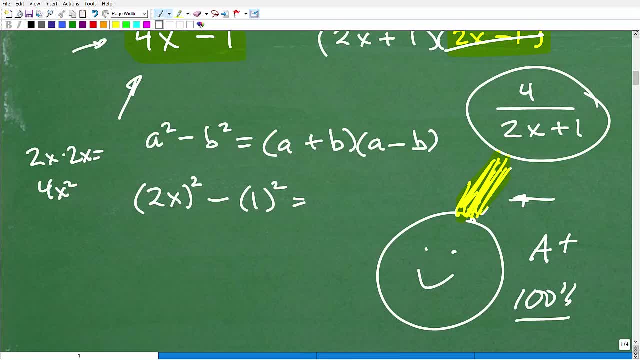 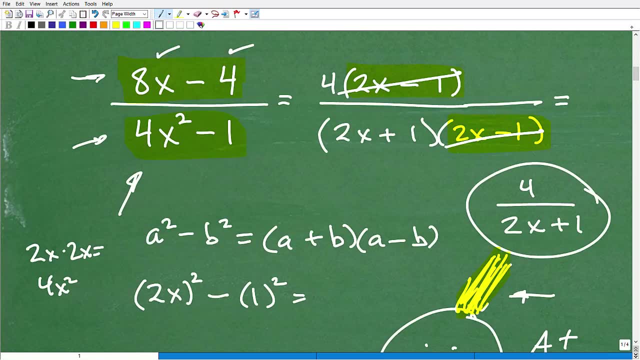 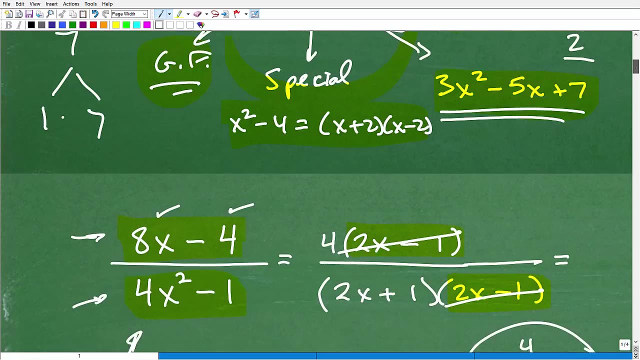 and a 100, so very, very good. now I will say that this was a pretty easy problem, okay, when it turned in terms of factoring. there's much more difficult problems dealing with trinomials and everything else, but it shows me that you're on the right track, okay, but again, all right. what you want to do is really 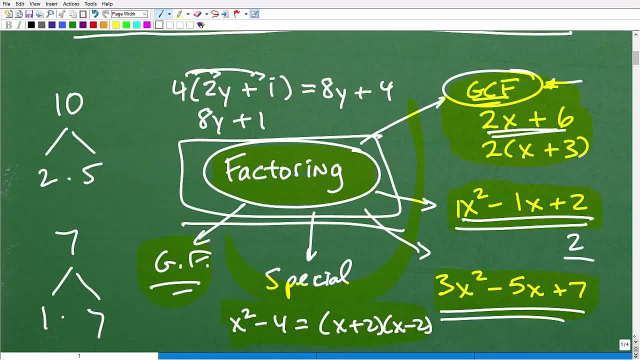 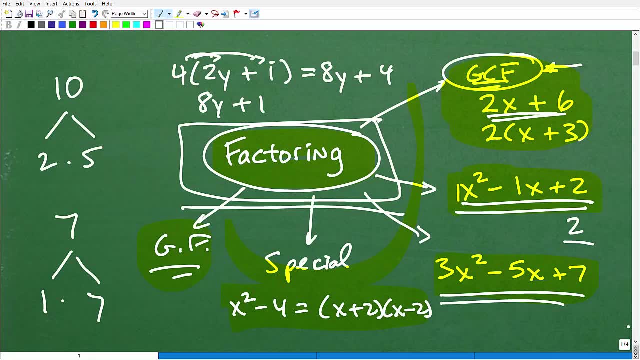 take an assessment of your current factoring skill sets and be like: all right, we're doing. is there anything I'm missing here? because if you strengthen this skill, this is a critical skill and it's not only just an algebra one. if you have any intentions, I don't know where you're at in your math courses, but 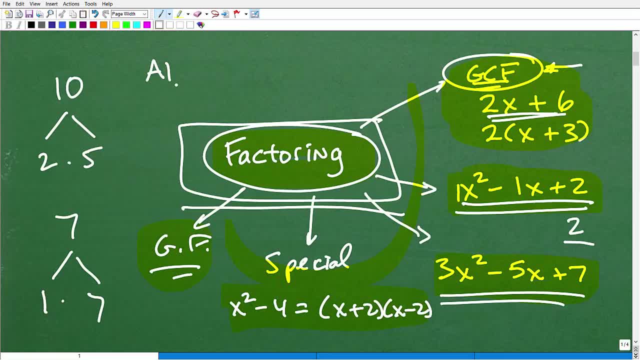 this stuff is just going to continue on. so whether you're taking algebra one or pre-algebra, let's just back it up here. pre-algebra goes to algebra one. you start learning a little bit of factoring. algebra one: factoring geometry. you use algebra in algebra two: tons of factoring, move on to 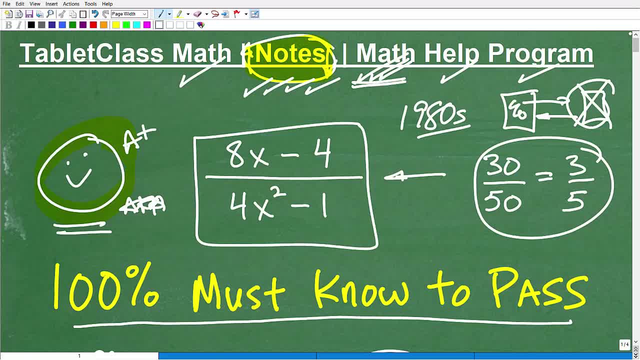 pre-calculus: massive amounts of factoring. so you know it's never going to go away, okay, so, uh, you know. anyways, hopefully I made my point about factoring. I don't want to, uh, sound redundant like the you know, extra, extra, extra redundant, but I know that's what, the way I'm sounding like a. 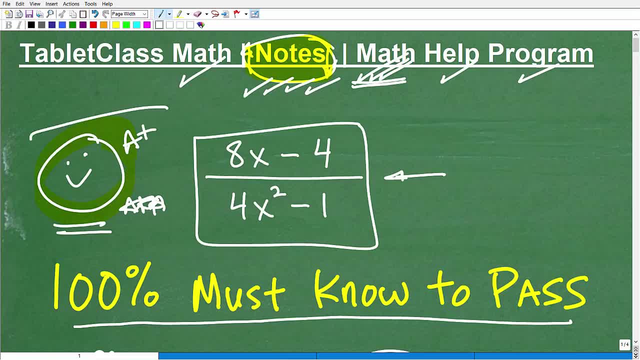 broken record, but it's that important, okay. so if you want to end up looking like this in your algebra course, master factoring, all right. so if this video was helpful in some small, tiny little degree, please consider smashing that like button. that definitely, definitely helps me out. and if 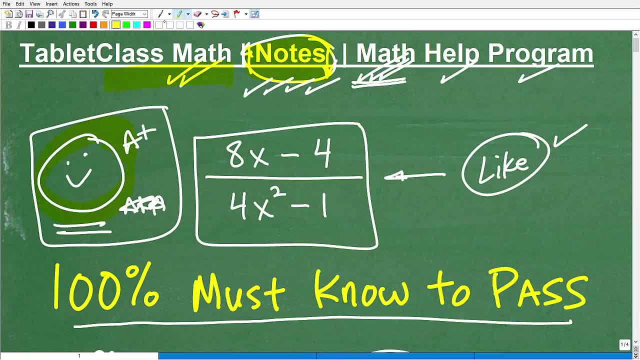 you're new to my youtube channel, please consider subscribing. I've been on youtube for 10 plus years, have over a thousand plus math videos ranging from basic to advanced math on my channel- all there for you. so if you like my teaching style, please take advantage of all these videos and all the new stuff. 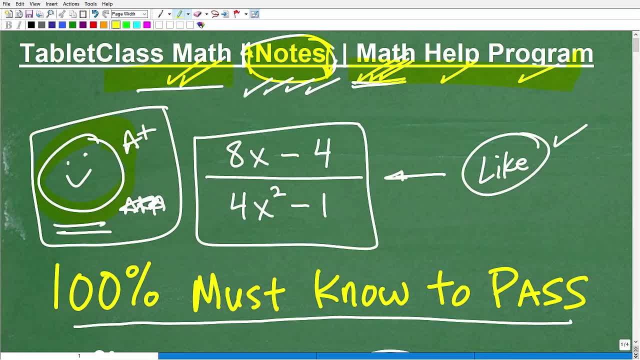 that I will be doing in the future, but my best math help will be within my math help program, okay, so, with that being said, I definitely wish you all the best in your mathematics adventures. thank you for your time and have a great day.